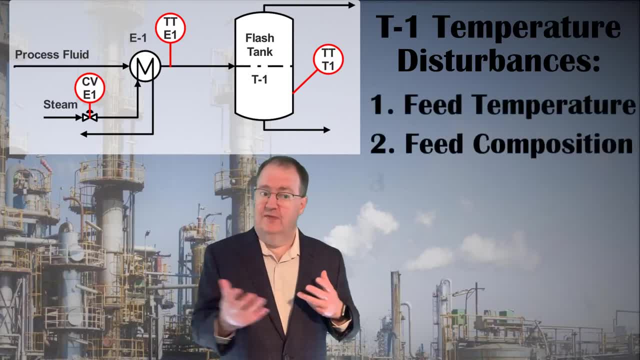 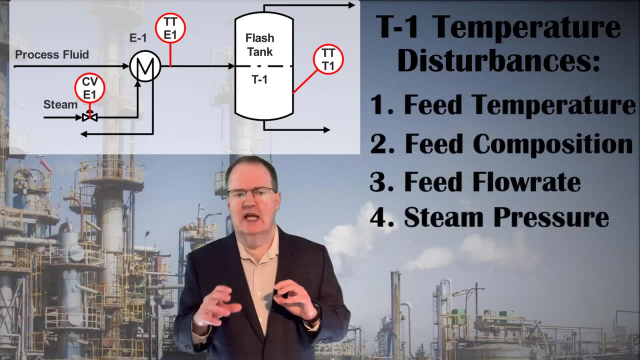 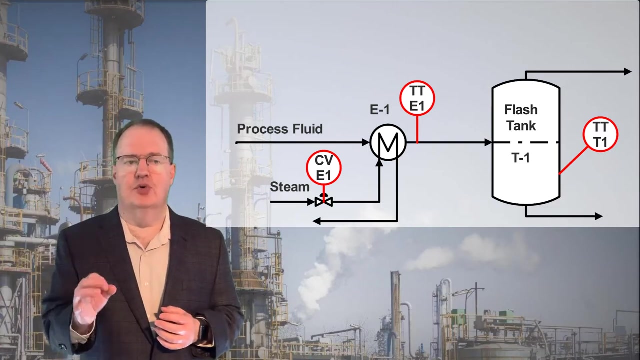 The feed temperature, the feed composition, the feed flow rate or the steam pressure. The interesting feature of each of these changes is that they would all affect both temperatures: the fast TTE1 as well as the slow TTT1.. The improved solution to this problem is called a cascade control scheme We're going to implement 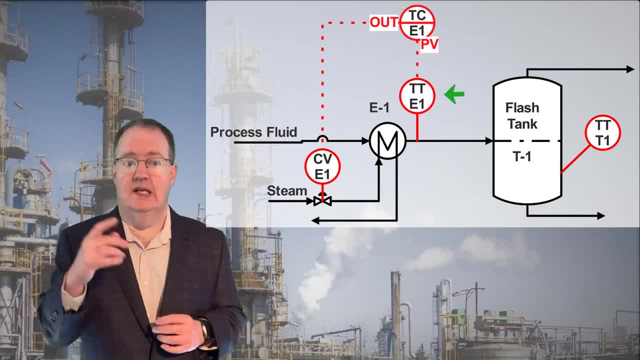 two controllers. First, we're going to control TTT1 and TTT2.. We're going to control TTT1, the exit temperature from the heat exchanger, which will be a fast loop, by manipulating the steam valve with the controller TCE1.. 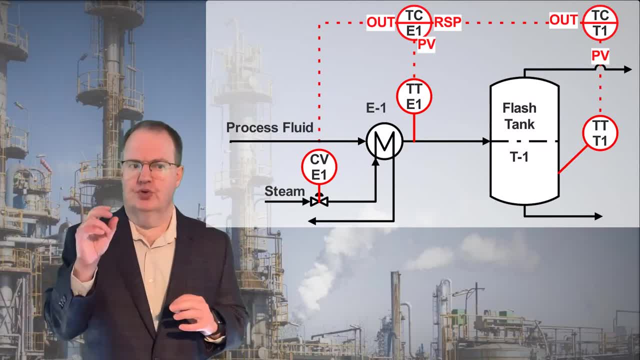 The second loop with the slow dynamics will control TTT1 by manipulating the set point to the first controller, TCE1.. When T1's temperature is low it raises the set point for TCE1.. That controller will react to an increased target set point. 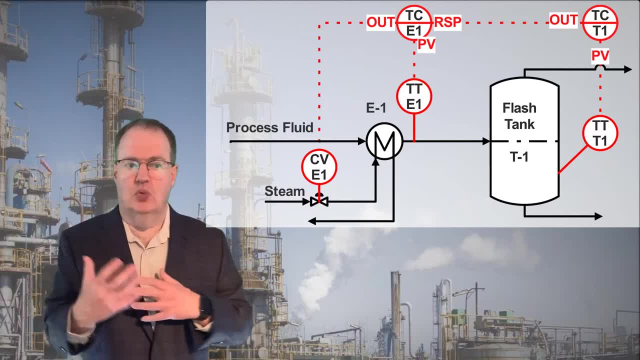 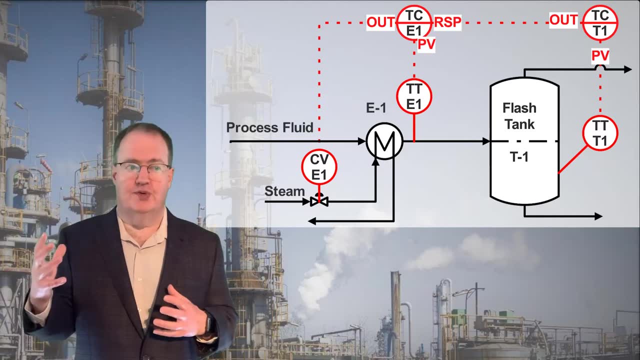 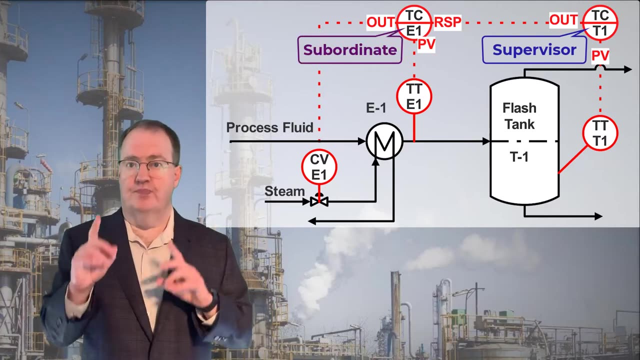 for TTE1 by manipulating our 1 degree of freedom to steam valve. We're going to label TCT1 the supervisory controller, because it is giving commands to TCE1, which we will call the subordinate controller. In a cascade steam, the subordinate controller is: 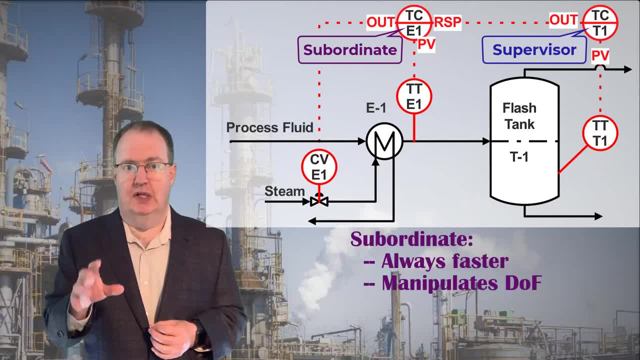 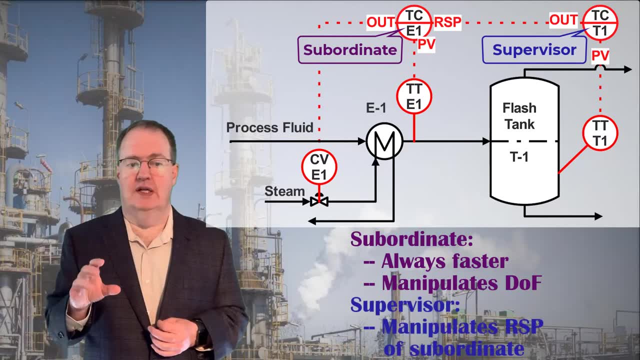 always going to react. In fact, they do react. together followed svd banks in the Scholar the fast loop, and always manipulates the degree of freedom, the output of the supervisory controller, always manipulates the set point of the subordinate controller, which we label rsp. 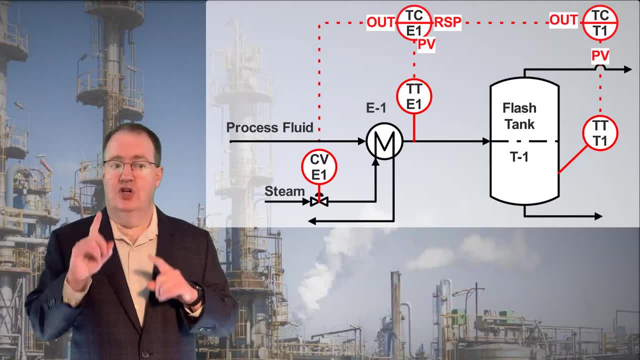 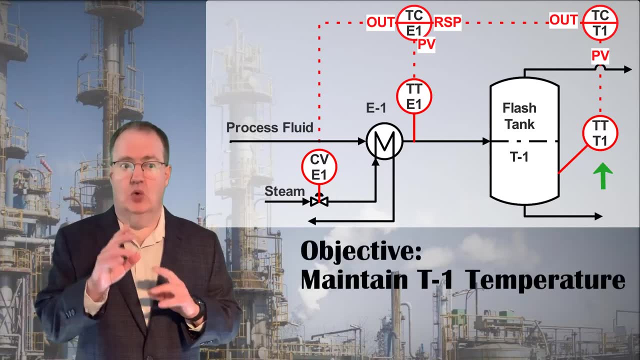 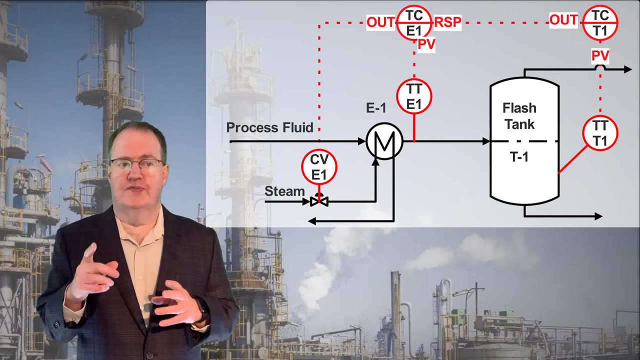 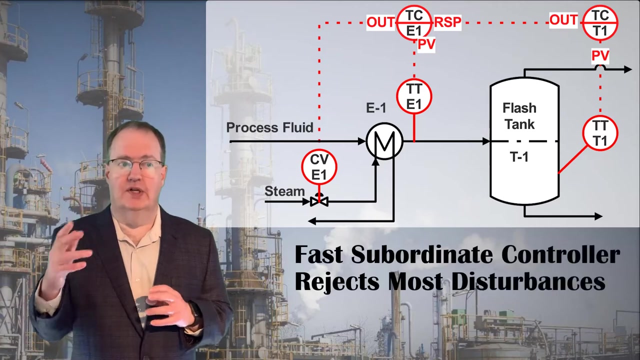 for remote set point. note: we have not created an extra degree of freedom here and we're still only satisfying one objective and manipulating one valve. but a cascade control scheme has multiple advantages. first of all, all of the disturbances that we listed affecting ttt1 will affect tte1 as well, but they affect the subordinate temperature much faster, and the fast 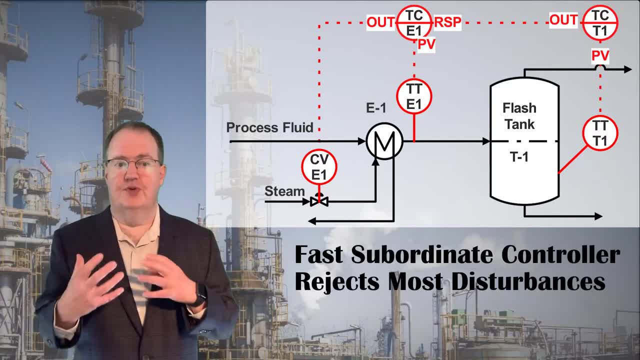 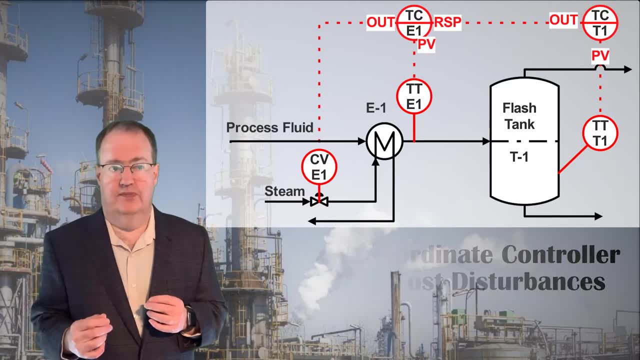 subordinate controller will adjust to reject those disturbances on the secondary objective with little or no effect on the subordinate controller. and the fast subordinate controller will adjust to reject those disturbances on the secondary objective with little or no effect on the primary objective. next, the subordinate controller can be operated. 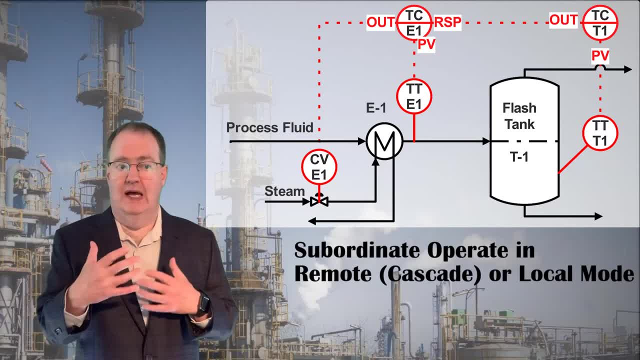 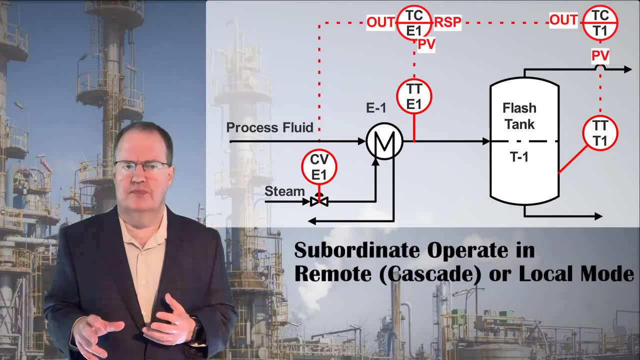 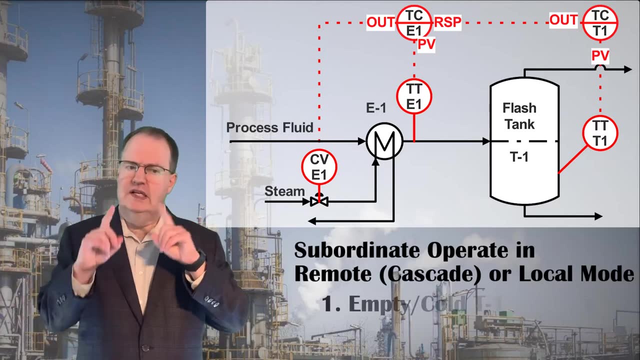 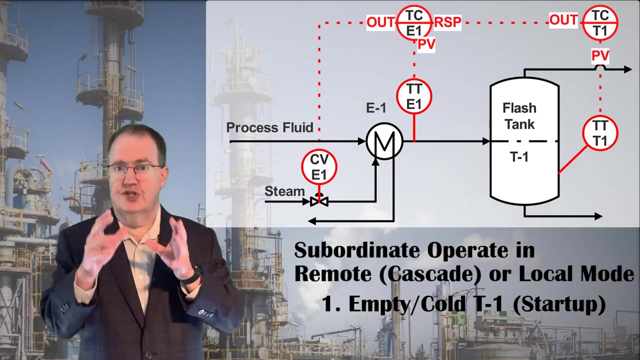 in cascade or remote set point mode, as drawn, or it can be switched to local mode, where it ignores the supervisory controller. now why would we allow this act of rebellion against the supervisor? well, when t1 is starting up and empty, it would be better to run in local mode that is just controlling the exit temperature of the. 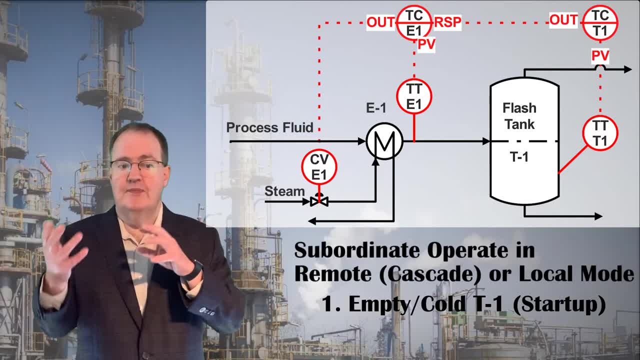 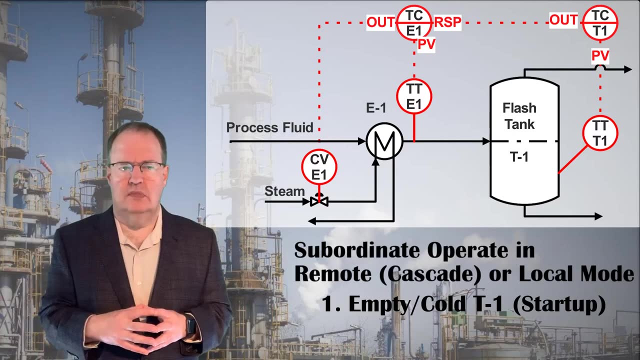 heat exchanger and ignoring the t1 temperature until t1 fills and heats up, because otherwise the supervisory controller might call for too much heat early on, overheating the fluid or causing an overshoot in the temperature. local control would also allow temporary operation if tt t1. 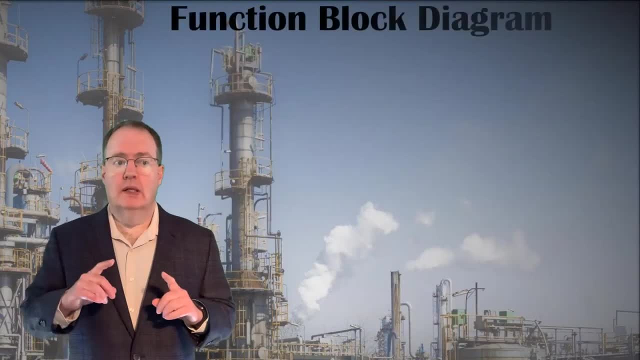 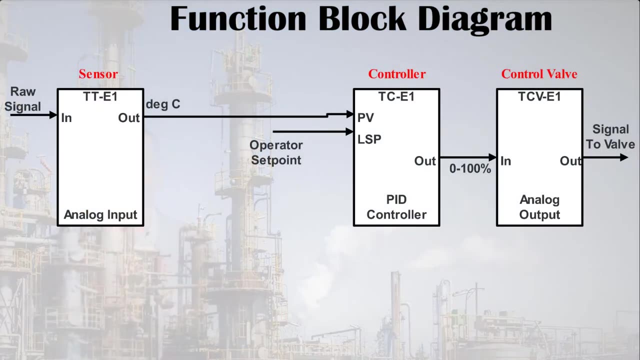 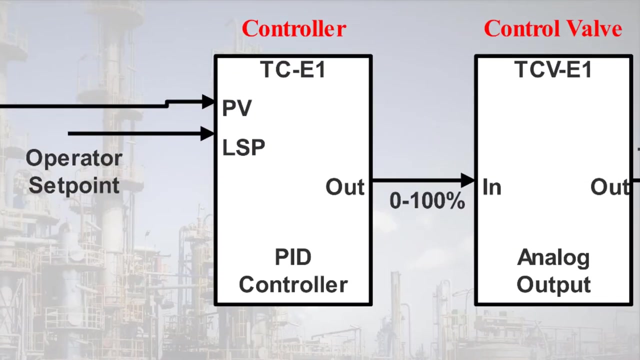 malfunctioned. at this point, let's introduce the function block diagram, or fbd. fbds represent the elements of a control loop, such as sensors, valves and controllers with rectangles called function blocks. each function block exists in the control system and each carries out one task. inputs to a function block are on the left and outputs are on the right. 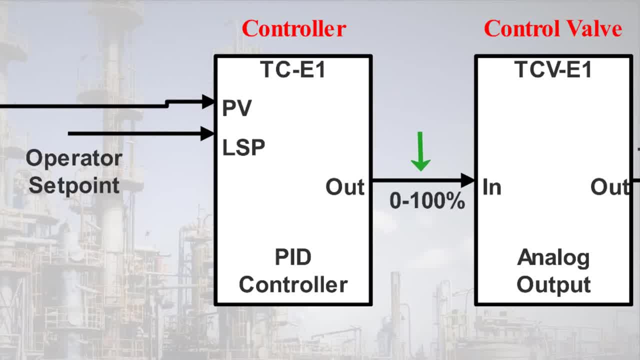 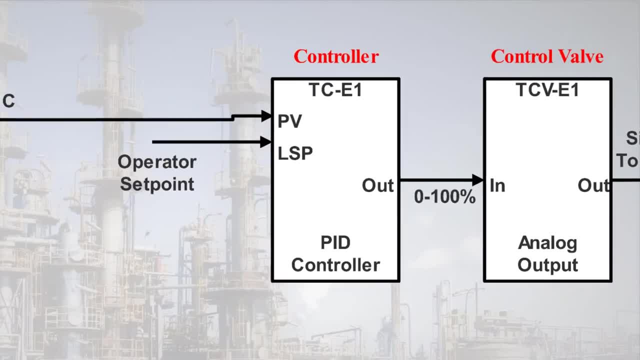 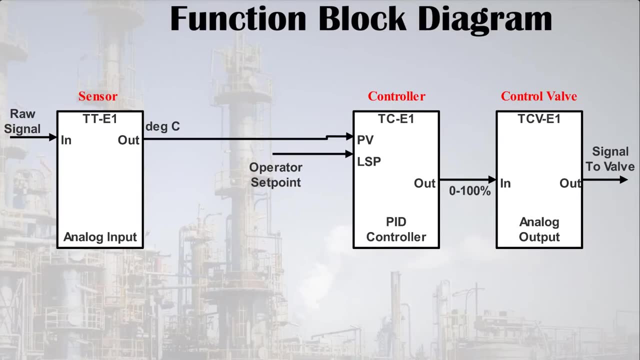 the lines connecting the blocks represent signals which we often label with their units. fbds are a useful visual tool and continuous controls on most programmable logic controllers or distributed control systems are configured using interactive fbd displays. so you'll see fbds in the workplace here on the left we see the temperature transmitter tt t1. 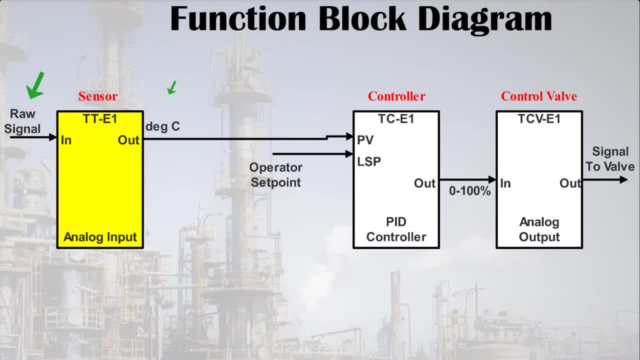 converting a raw signal from a sensor to a signal in degrees c. that signal becomes the process variable or pv of the controller tce1, which also receives a local set point. the controller's output of zero to one hundred percent goes to the function block for cv e1, which converts it to an electrical signal. 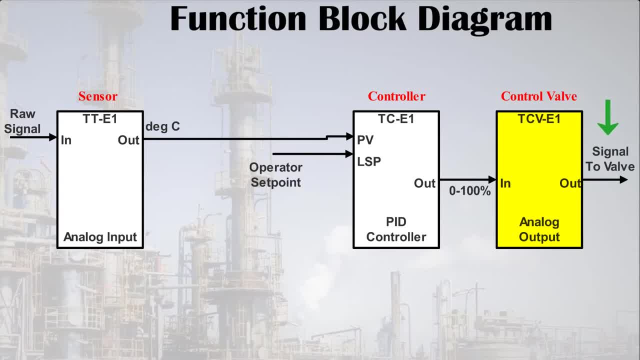 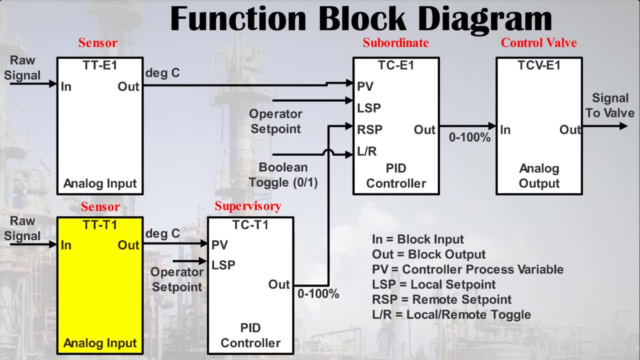 to the valve. this is our subordinate loop. when we bring in the components of the supervisory loop, we have another sensor input, ttt1, and another controller, tct1. the output of the supervisory controller tct1 becomes the remote set point for the subordinate controller tce1, just as we did when we were 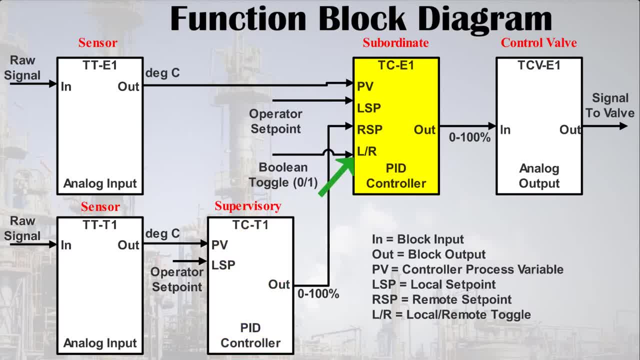 diagramming this as a p and id. and on tce1 there's now another input for that controller which allows it to be toggled between local mode l, where it ignores the supervisor, and remote or cascade mode r. boolean toggle just means one or zero on or off. we'll be using the fbd often. see more examples in: 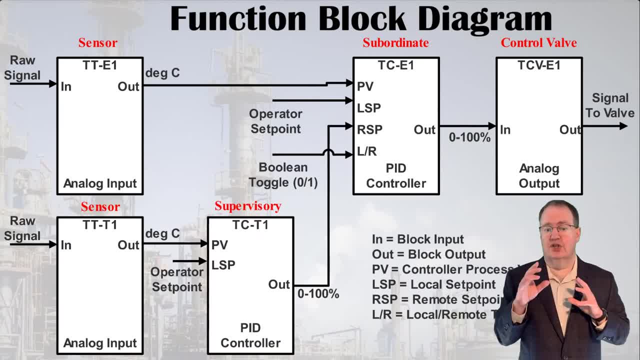 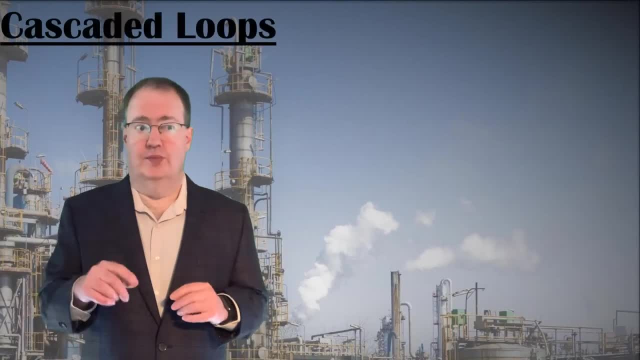 the text. also in the text see another good cascade layer as we move forward with a simple notifications. but your cascade design example for reflux control of a distillation column, Do the cascade exercises at the end of the chapter to get used to this commonly used technique. A brief note on terminology. 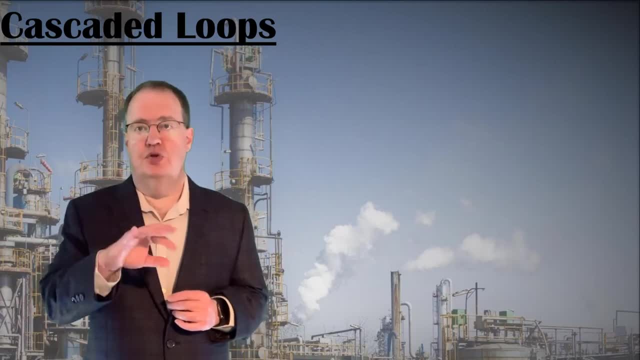 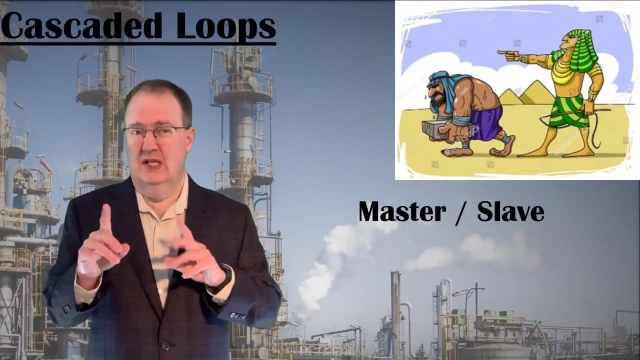 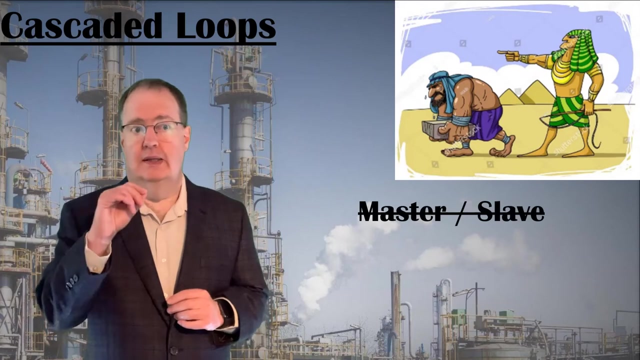 From the point they were introduced. until recently, the two cascaded loops were referred to as the master and slave loops. Now, do we really need or want to reference human bondage to convey the meaning intended? Clearly no. A lot of other sources currently use the labels primary loop. 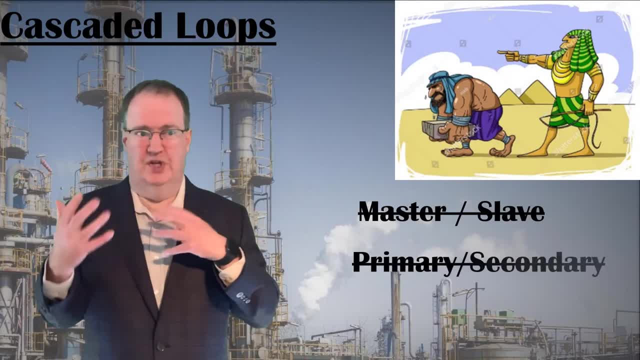 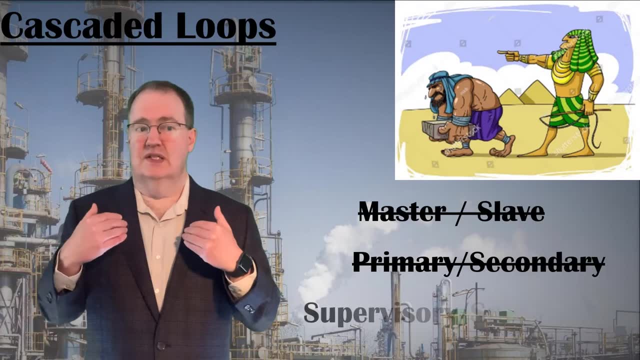 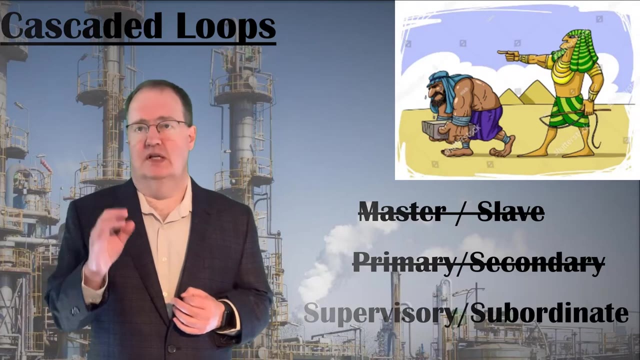 and secondary loop, but I can never remember which is which. Supervisory and subordinate is my preferred terminology because it describes the design clearly and because I made it up. Be warned that you'll see other terms in other places. Our second topic in this chapter is the design of the design. 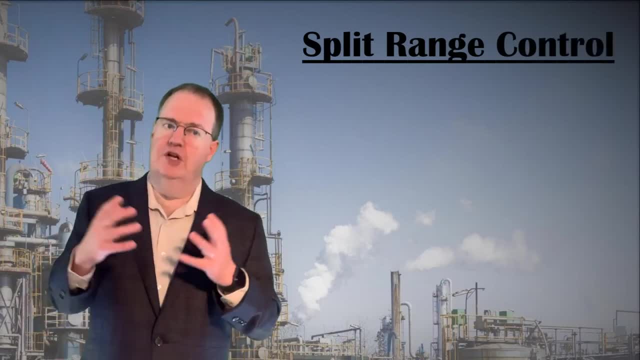 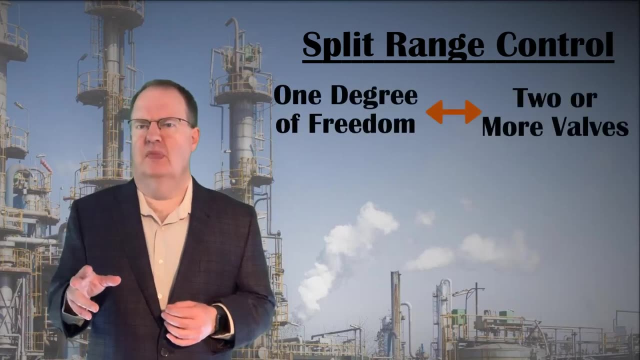 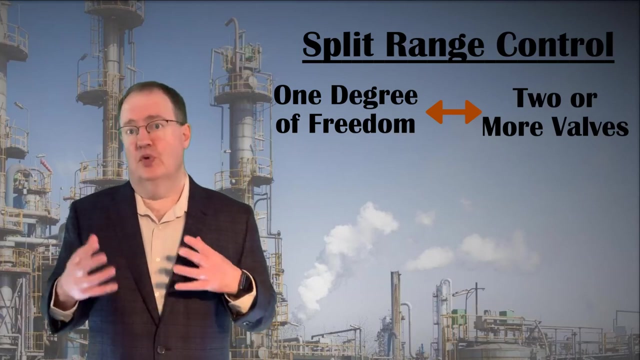 This video is split range control. Split range control is necessary when we need more than one valve to control one degree of freedom. Now, why would we need that? Well, largely, these applications fall into two groups, both of which are quite common. The first is where we need two. 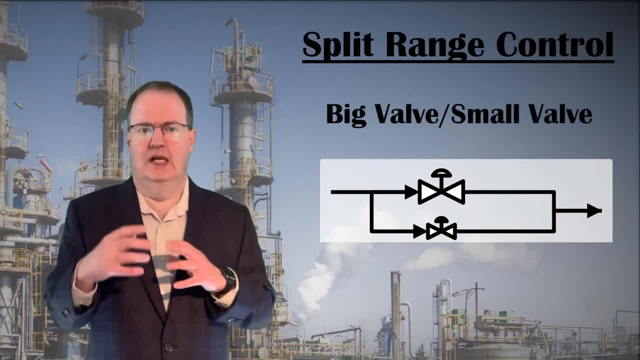 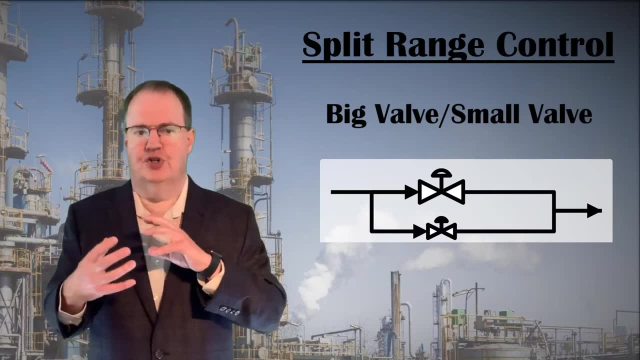 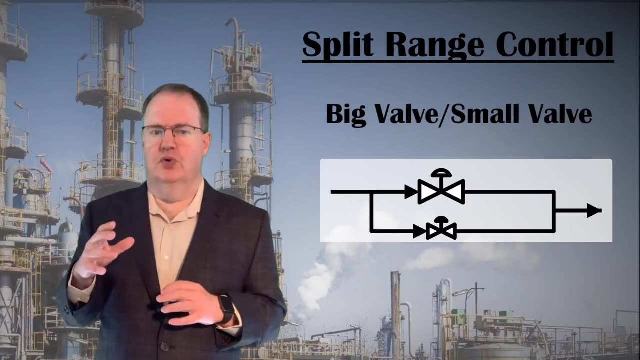 different size control valves to operate at two different operating points. Control valves are based on a flow rate and a pressure drop due to fluid properties And when the process, often a batch process, needs a flow to be controlled over a wide range of flows or properties, one valve: 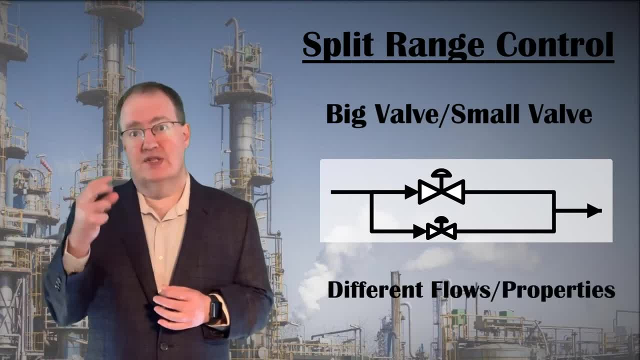 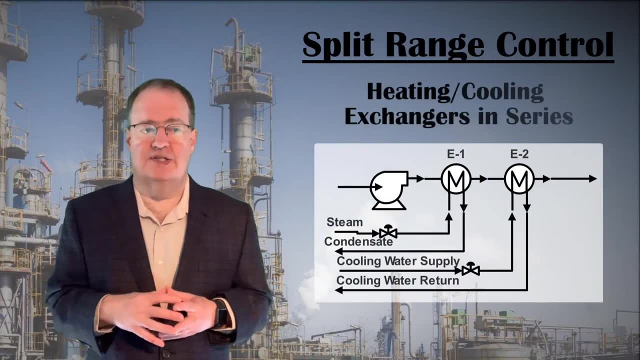 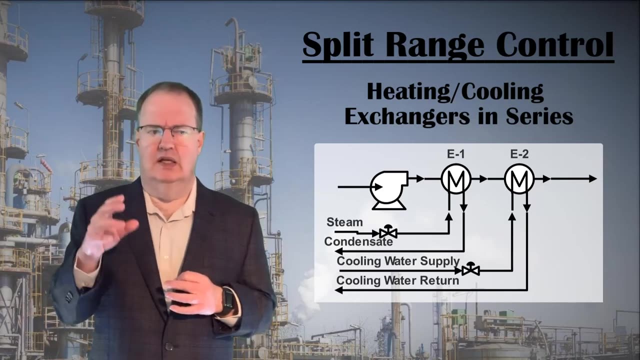 can't satisfy the whole operating range, So we install two valves in parallel, one big, one small. The second case is when we have a design where one process stream needs to be heated in one set of conditions and cooled in another, So the stream is put through two heat. 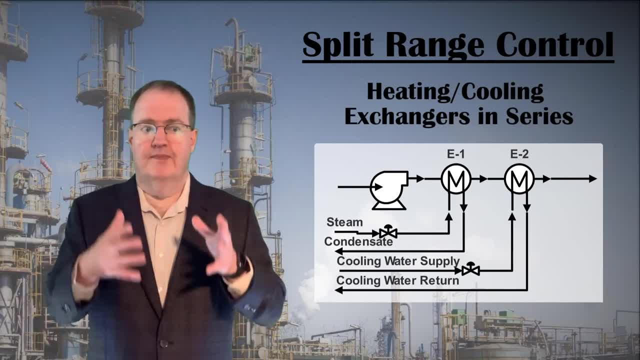 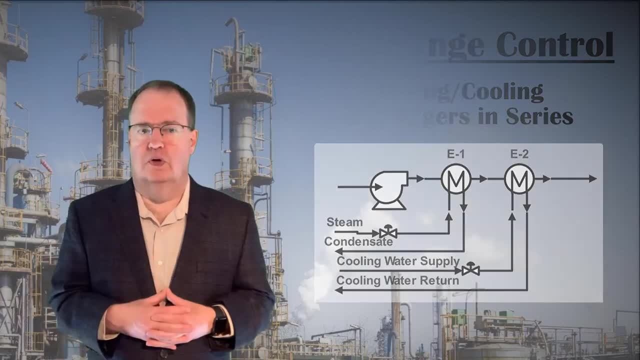 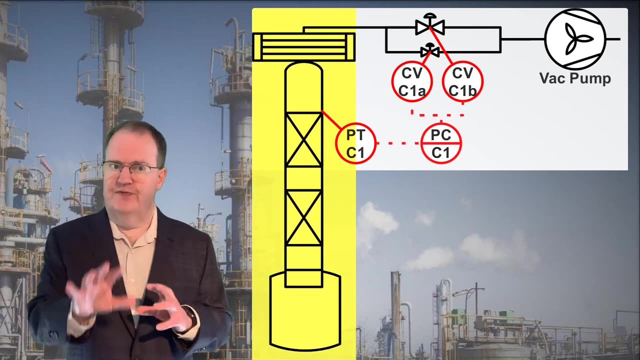 exchangers: one for cooling, one for heating, each with its own control valve on the two utility flows, the hot flow and the cold flow. Here we see an example of the first. C1 is a batch column that operates under vacuum, The small valve, CVC1A. 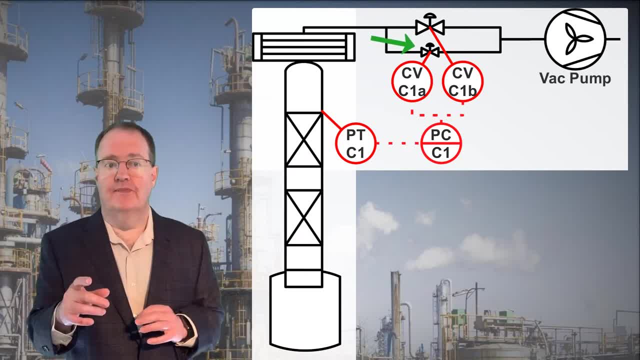 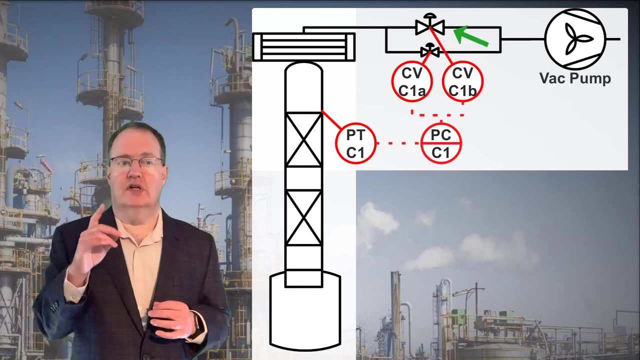 is used to control pressure close to atmospheric, But as the pressure decreases and the vapor density falls, CVC1A is no longer big enough and the larger CVC1B is needed to control pressure. We need to convert the output of the controller PCC1, to appropriate signals for the two valves. 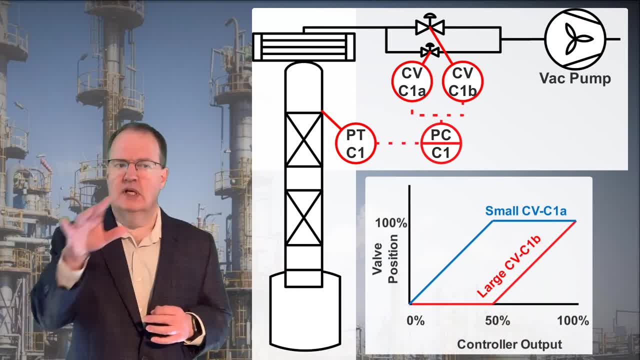 as shown in this graph, The x-axis is the controller output And the y-axis is the signals to the two valves. In blue we see the small A valve open from zero to 100 percent, as the controller output ranges from zero to 50 percent. Above a controller: 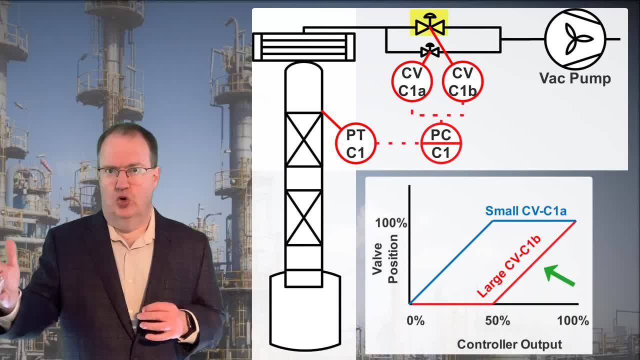 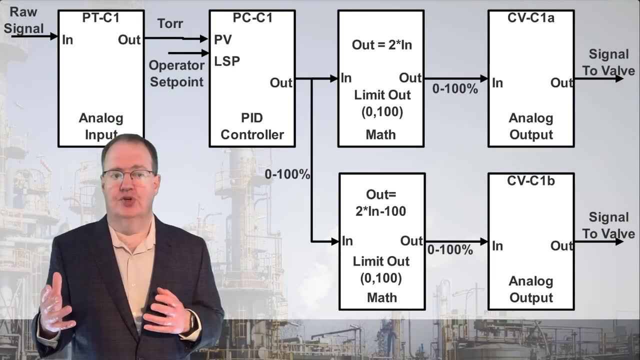 output of 50 percent, CVC1A is wide open and CVC1B, in red, starts to open from zero to 100 percent. as the controller output increases from 50 to 100 percent. The function block diagram for this solution.